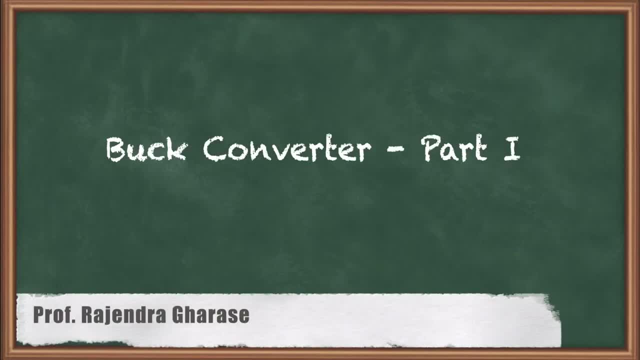 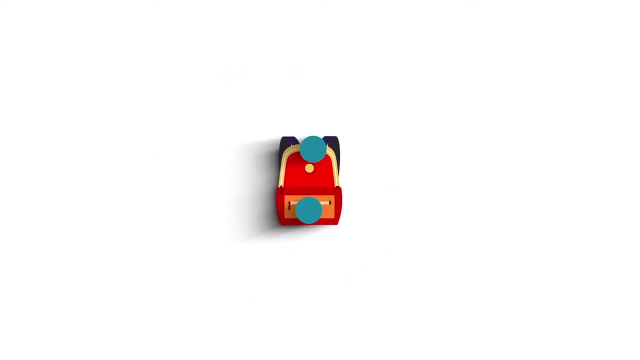 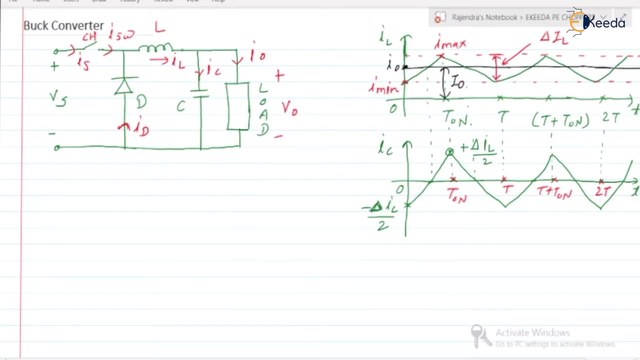 Hello, friends, in this video we are going to discuss about the buck converter, the circuit operation. Okay, So here we are having the circuit diagram for the buck converter. Here Vs is the supply voltage, which here we are having. that is nothing but the chopper, the 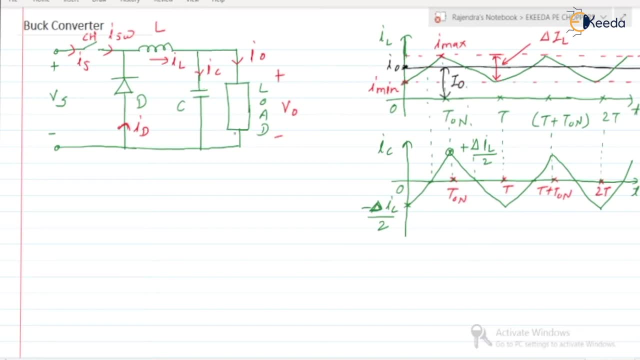 diode inductor, capacitor. and here it is a load. Okay, Here, if you check, if you compare this circuit with a step down chopper, Okay, Here we have added a diode inductor and a capacitor. Okay, Next, voltage across load is V0, current flowing through the load is: 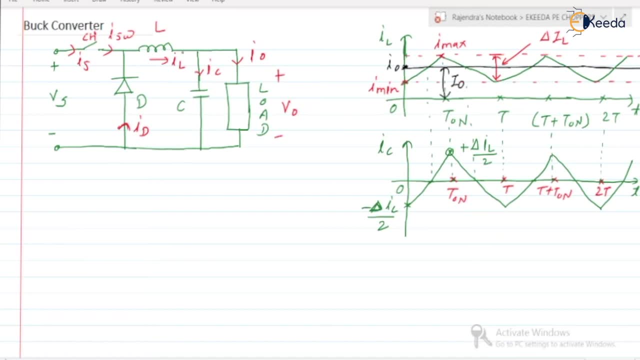 I0.. Current flowing through the capacitor is Ic. Current flowing through the inductor is Il. Current flowing through the diode is Id. Right. The supply current is Is. Switch current is Isw. Okay, Now let us discuss the circuit operation. Okay, So here, when, 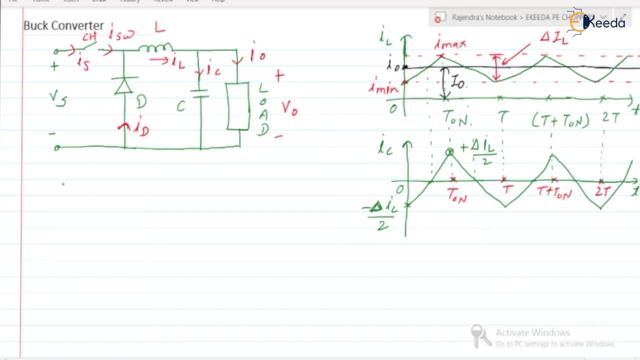 switch is in the on state. when switch is in the on state so we can write during: during T is equal to 0 to T on T is equal to 0 to T on Right. So during T is equal to 0 to. 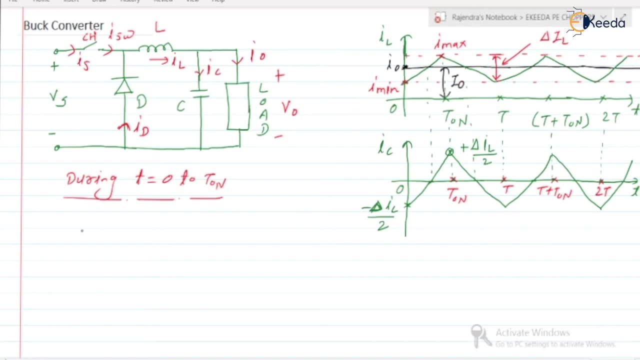 T on. Yes, that is, switch is in the on state. Okay, So when switch is in the on state, at that time what will happen? The circuit like which is acting as a short circuit. here we have capacitor Next load. 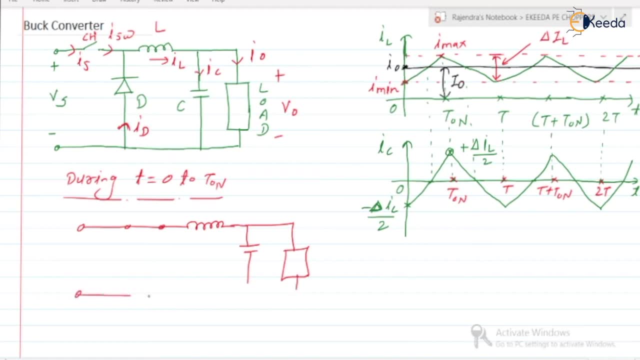 Okay, And the diode will be in the open state. Right, Because diode will be in the reverse bias mode. Okay, Because when switch is in the on state, the diode will be in the reverse bias mode. Okay. So at that time, if you check, yes, this is the load we are having, Okay. 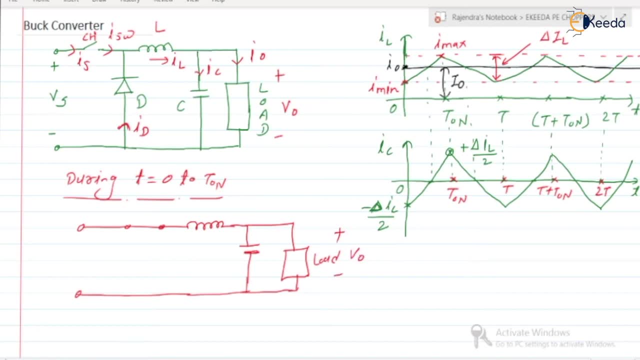 Voltage across load is V0.. Right Next capacitor. Capacitor current is Ic. Okay, This is the I0.. Inductor: L Inductor current is Il. Okay. Inductor voltage is VL. Diode is open circuit. 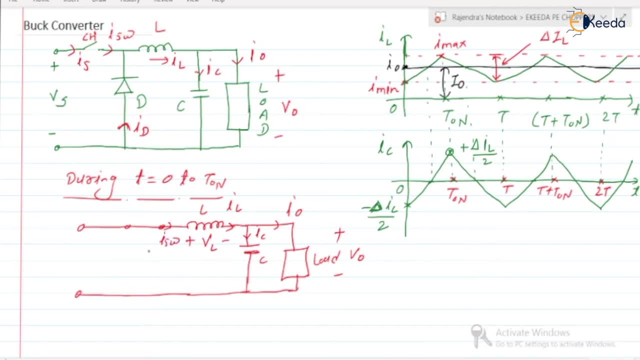 which is closed. Right, So this current is Isw, This current is Is: Okay, And here we are having the Vs. Okay, So it is like when switch is in the on state. Right, So this is the on state Inductor. go on storing the energy. Okay, So here in all the converters. 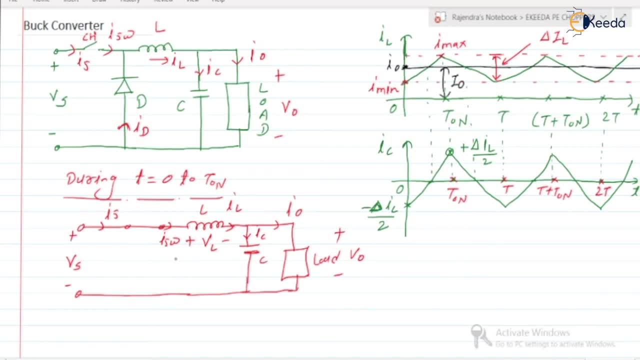 buck boost or buck-boost converter. Okay, We are going to assume that the load voltage is constant. Load voltage is constant and the load current is also constant. Okay, So here, load current. I have assumed it is a constant. Okay, So what are the assumptions? Load current: 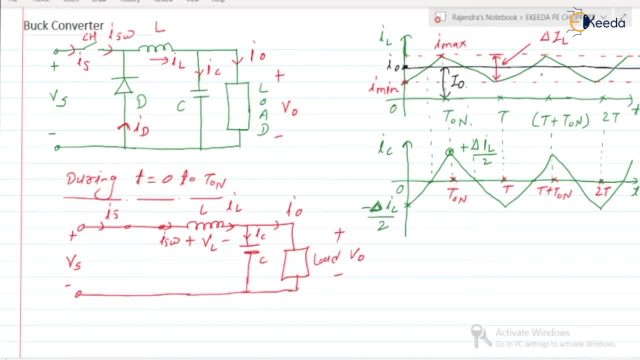 is constant and, at the same time, load voltage is also constant. It is a ripple free, Okay, Because if you check, if you check in the case of step down chopper, yes, what was the V0? V0 waveform was? it is a like non Vs, after that zero, after that again Vs, like this waveform. 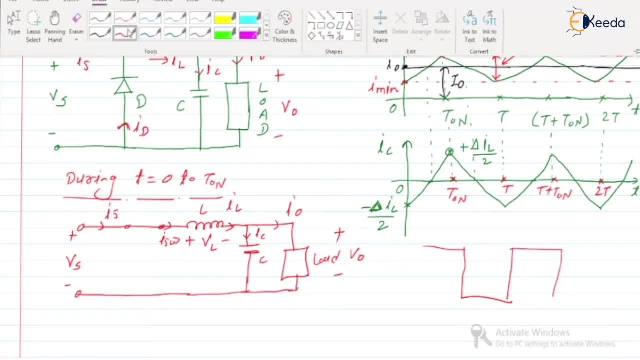 we were having. Okay, So here, in order to avoid that waveform. yes, here we have connected a inductor, a diode and a capacitor in a circuit. Okay, So, due to that, what will happen? Yes, Here, if the switching frequency is increased, then we will be getting the constant load. 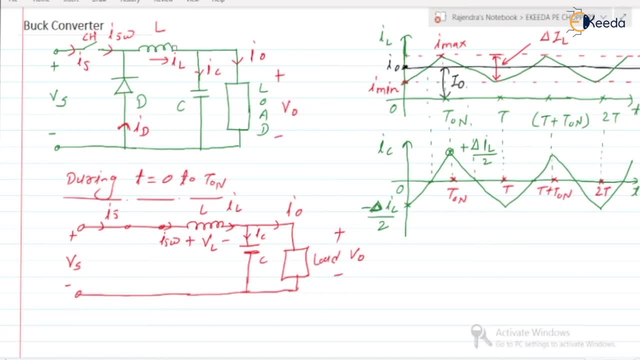 current and the constant load voltage. Okay. Now the function of the inductor is it acts as the change in the current. Okay, So that's why it will cause the current flowing through the load to be constant. The function of the capacitor is to oppose the change in the voltage. Okay, 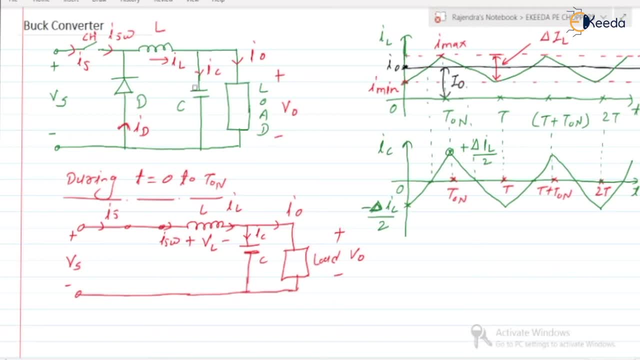 So that's why the capacitor is connected across the load, So that's why this capacitor will try to maintain the constant voltage across the load. Okay, So now, when t is equal to zero to t1か, when t is in between zero to t1か, okay, at that time we will be having 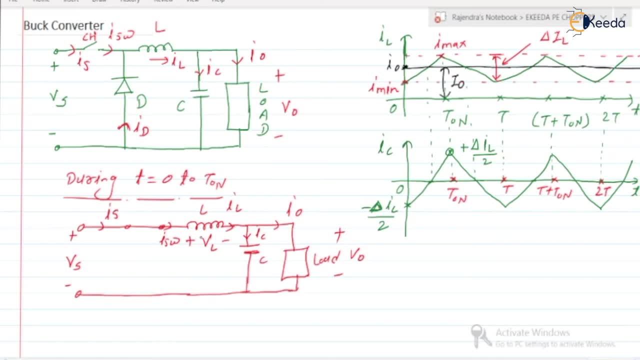 yes, during this time will be having. inductor is storing the energy. inductor is storing the energy. so now, coffee represents this temperature. Yes, IT is turning on Now, if the capacitor is turning on and off. Okay, carcinogen andlicium, which means that the sheet pressure. 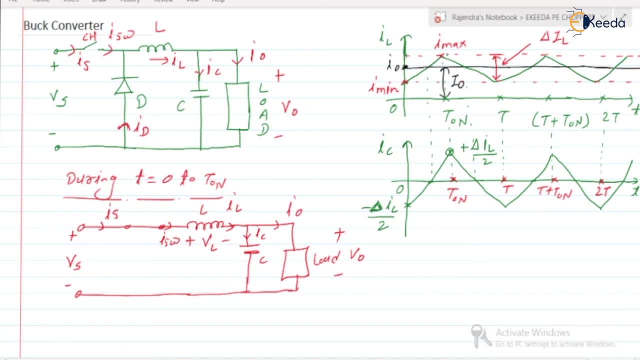 So inductor current will be increasing from I min to I max. For very first cycle it will be starting from 0. But for continuous cycle it will be starting from I min to I max. okay, So inductor go on storing the energy. right Inductor is storing the energy. Next, as I said, I0 is. 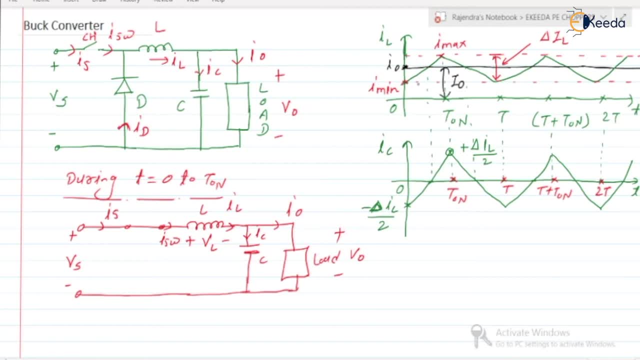 constant current right. I0 is a constant current. I0 means what It is: average of I min and I max. average of I min and I max. okay, So I0 is a constant current. Next here, if you check: 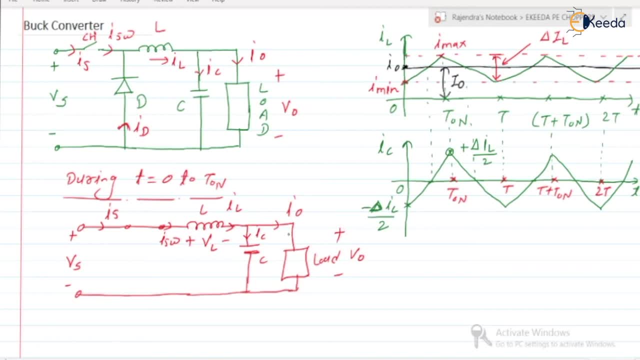 right, IC is equal to what IL minus I0.. Yes, we can write IC is equal to IL minus I0, okay, But I0 is a constant current, So we can write it as a IL minus capital I0.. It is a constant load. 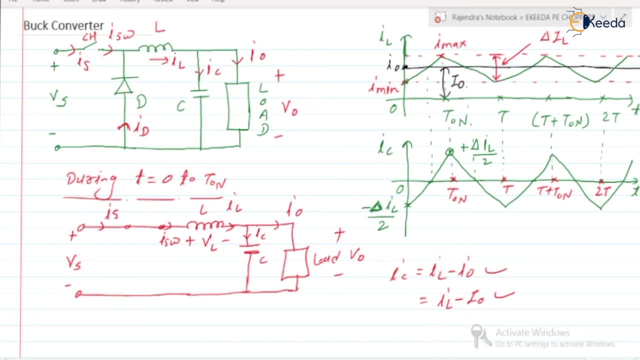 current. okay, So what is the IC? If you check when IL is I min, when IL is I min at that time, what is the IC? IC is IL minus I0, right, So it should be negative, right, Because I min minus I0,. 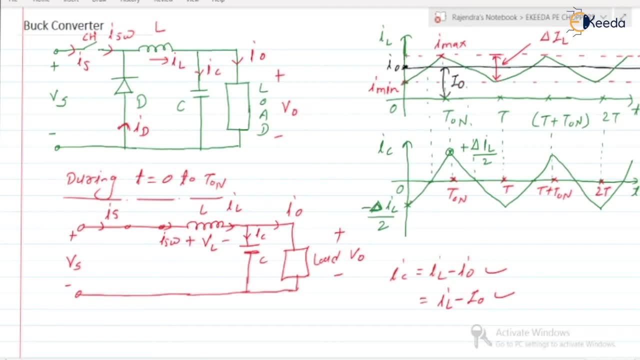 I min minus I0.. I min is less than I0.. So, therefore, it will be negative right. And what is the value of this? Yes, if you check, yes, it is this magnitude that is a delta IL right. Delta IL is nothing but. 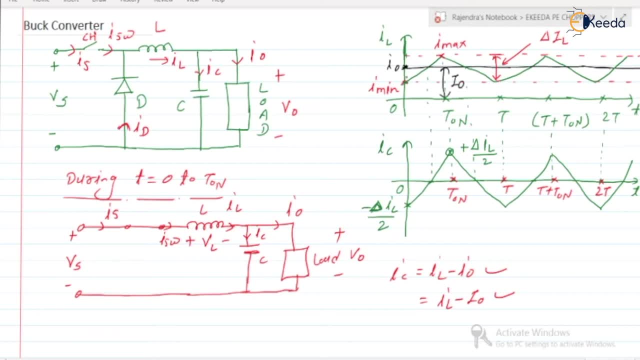 I max minus I min. okay. So can we say that this difference I min minus I0 is nothing but what? 50 percent of this delta IL? okay, So here we can write it as is equal to: yes, it is I min. 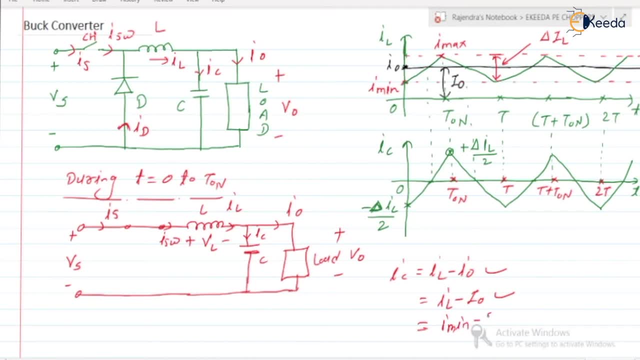 At this instant I am writing: okay, At this instant it is I min minus I0.. Right, So it is equal to what Delta IL divided by 2, okay, Delta IL by 2, minus delta IL by 2, okay. 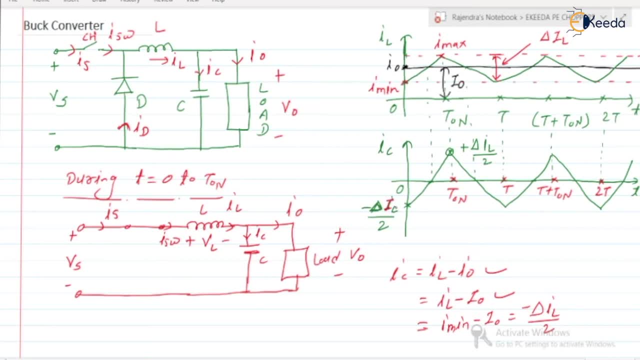 So if this IL is capital, yes, here also we need to take it as a capital. okay, So minus delta IL by 2.. Are you getting the point? Because delta IL means what I max, minus I min. This is the delta IL. 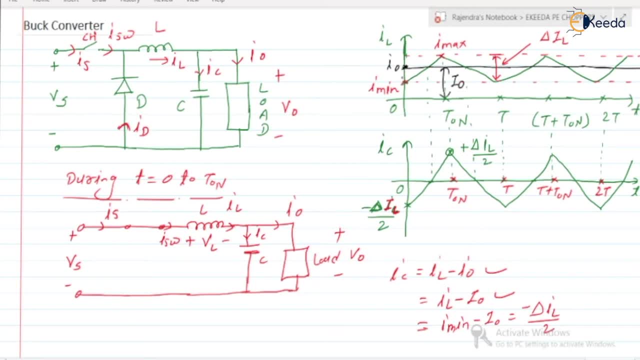 okay, So what is I min minus I0? I min is less than I0.. So definitely it is a negative. okay, And what is the difference? Yes, it is a 50 percent of this delta IL. okay, Next, so this is the minus. 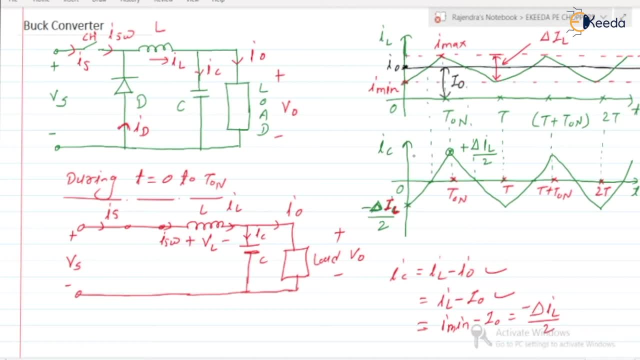 IL by 2, okay, So that is why here it is a we are having, I sin. So after that, as IL increases, this difference goes on decreasing. okay, At this instant, IL and I0 become same, equal So. 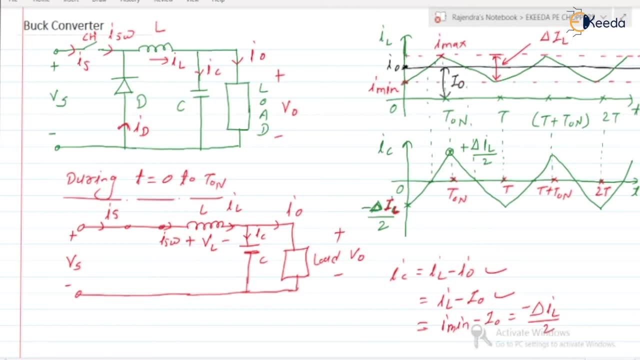 that is why the difference becomes 0. And after that, again, IL will be greater than that of the I0. So, again, this difference go on increasing. okay, And when IL is equal to at I max, when IL is equal to I max, at that time, yes, what is the value? When IL is equal to I max, then it is I max. 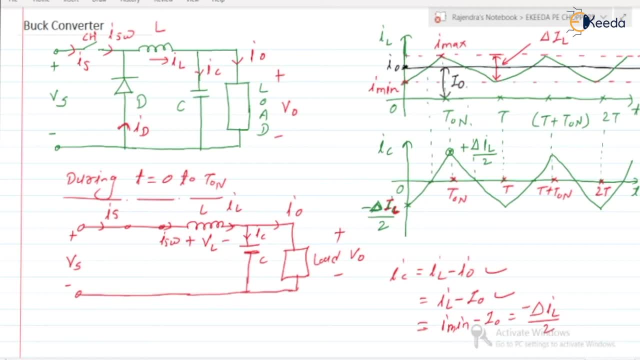 minus I0.. I max minus I0 is equal to I min, So this difference goes on decreasing, okay, So I max minus I0 means what? Again, I max minus I0 means 50 percent of this value, So it is a I max. 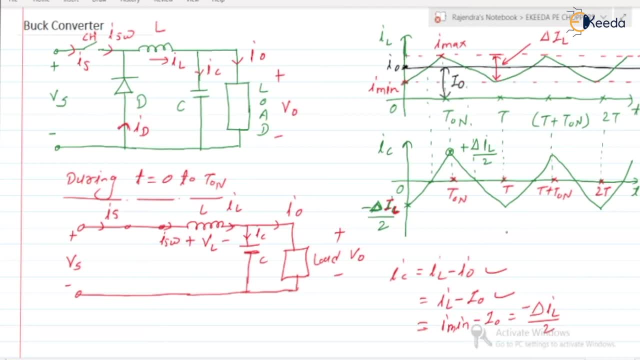 is greater than I min I0,. okay, I max is greater than I0.. So that is why it is a plus delta IL by 2.. So this value will be plus delta IL by 2, right? plus delta IL by 2.. Is this clear, Okay? 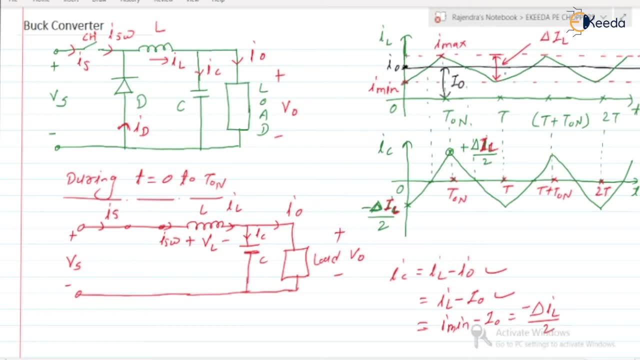 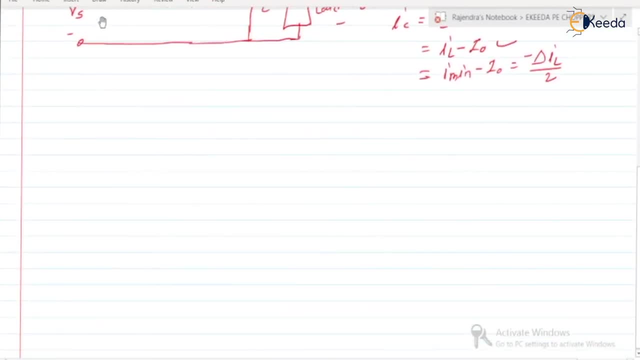 So in this way we can write: okay, After that, again during T on to capital T, during T on to capital T. what will happen? Yes, we can draw the circuit During, during T is equal to T- on to. 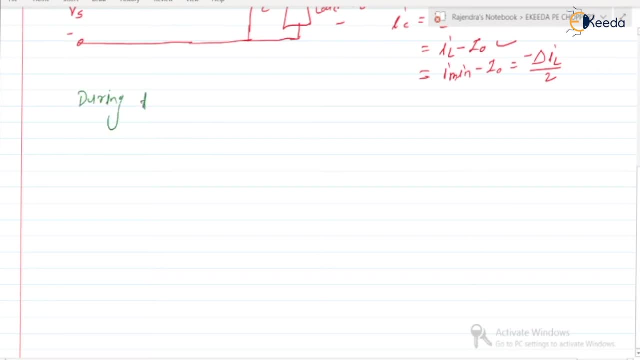 capital T. Yes, if you check, during this interval the switch is open. okay. So when the switch is open, the equivalent circuit will be like this, which is open circuit: Here we will be having the inductor, okay. Next, here it is a capacitor. Next load, okay. Next. here we will be having 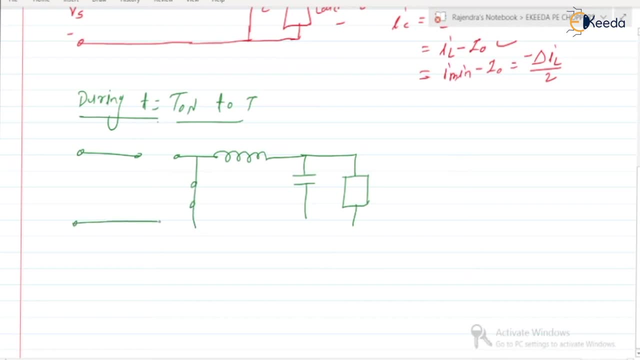 the diode That will be in the conduction mode. okay, So like this we will be having the circuit. okay, So load load voltage is V0,, load current is I0, okay. Next capacitor is a inductor: I0 current. this current is IC and this current is. 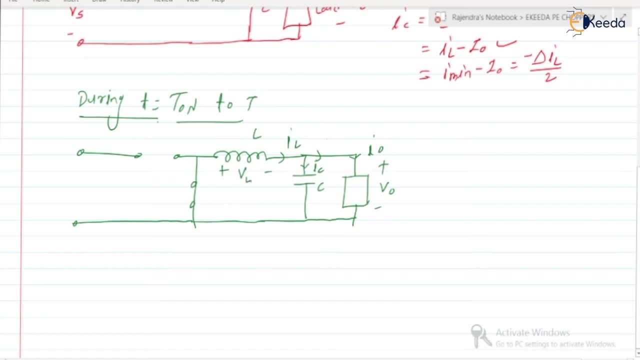 IL okay. Voltage across inductor is VL. okay, And diode current. here we will be having the ID right: Supply current is IS. Which current is ISW? okay, And this voltage is VS- right, This voltage is VS- okay Now. 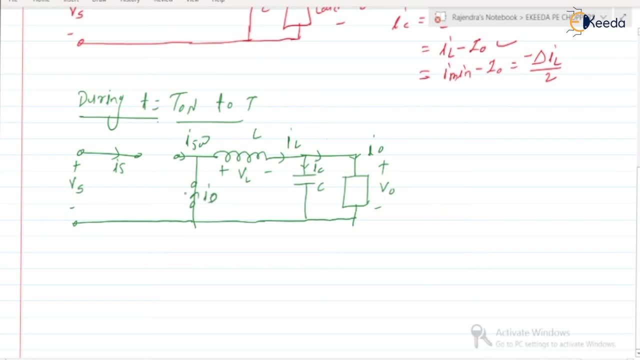 so if you check, if you check, yes, when switch is in the off state, that is, from T on to capital T, yes, whatever the energy stored by the inductor, inductor will release that energy. right, Inductor will release that energy through the load. Is this clear? Okay, So again, 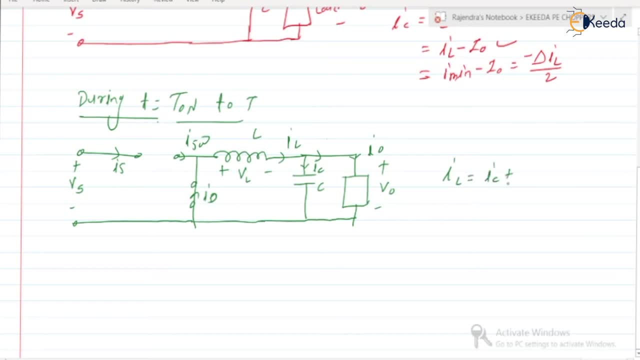 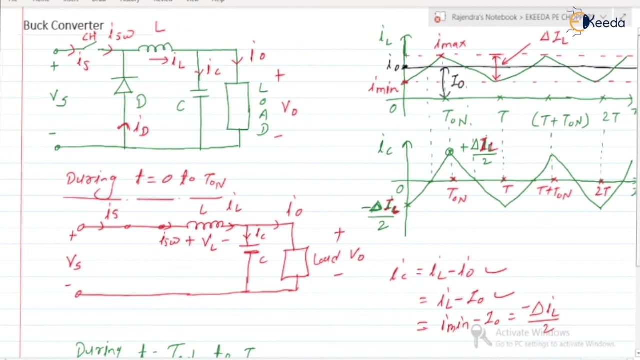 can we write it as IL is equal to IC plus I0, but I0 is constant current. So therefore IC is equal to what IL minus capital I0,. right, because of constant current. okay, So again, inductor is releasing the energy, means what Inductor current should go on decreasing. 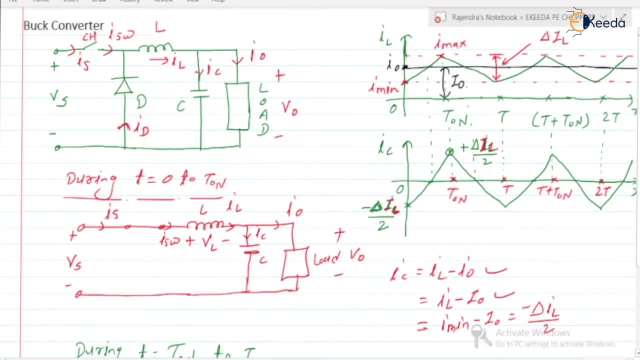 right. So inductor current decreases from Imax to Imin. Inductor current decreases from Imax to Imin. Is this clear? Okay, So when switch is in the off state, inductor releases the energy. So inductor current go on decreasing. okay, So as inductor current decreases, right, and it is. 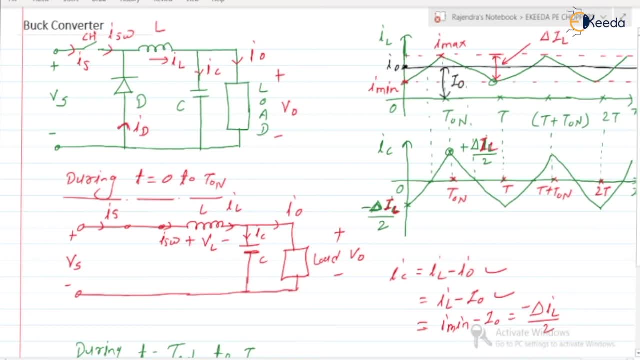 IC is equal to what IL, right, IL minus I0.. All right, So during this interval means from this point to this point, okay, IL is greater than I0.. So therefore, current or the difference is positive, okay. After that, yes, IL becomes less. 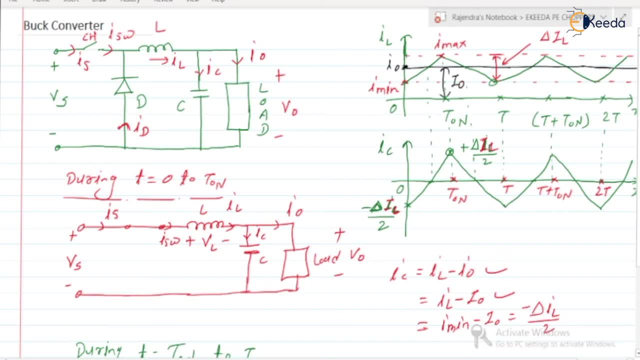 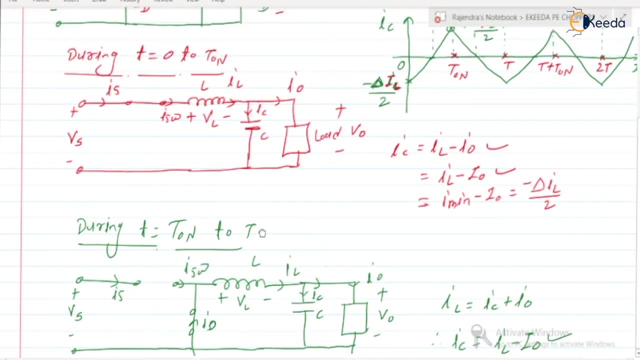 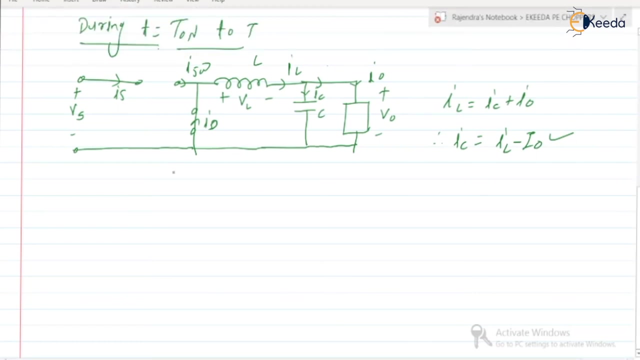 than I0.. So that is why the difference will be negative, That is, IC will be negative. okay, Next further, if you check- yes, if you check- during this interval, during this interval, what is VL Can you write? VL is equal to. during this interval, Yes, we can write VL. Apply KVL to. 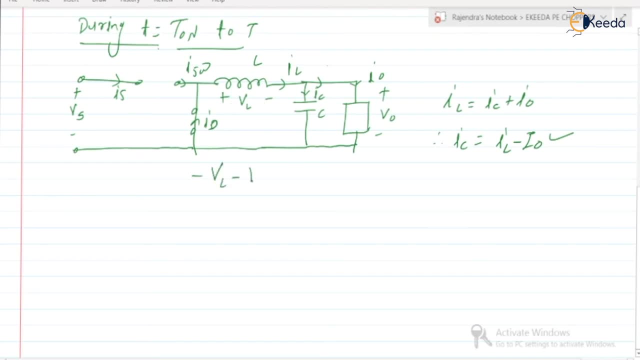 minus VL, minus V0.. We can write: minus VL, minus V0 is equal to zero. So therefore, VL is equal to what Minus V0,, right? VL is equal to minus V0,, okay. Next, during this interval, right during, 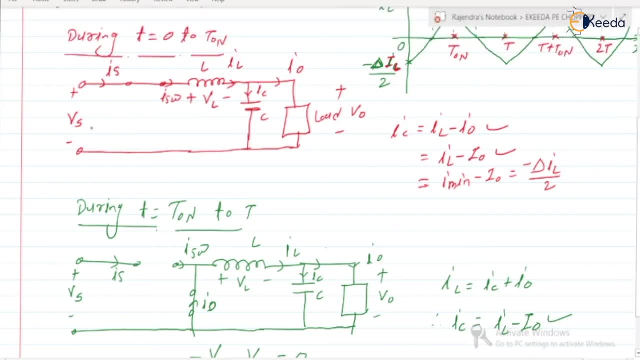 the during T is equal to zero to T1, what is the VL? Can I apply KVL? It is a plus VS minus, VL minus V0.. I am writing here plus VS minus VL minus V0 is equal to zero. So therefore, VL is equal to. 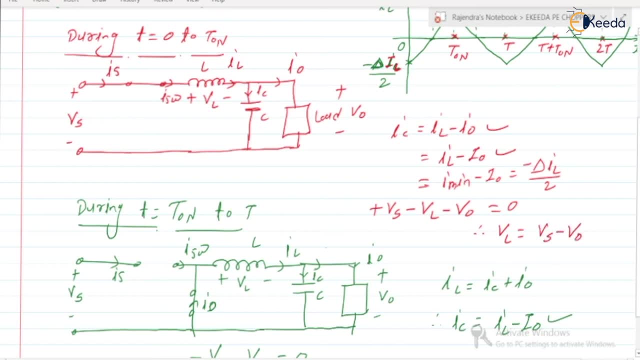 it is a VS minus V0, VS minus V0.. Is this clear? Okay, So this is during: T is equal to zero to T1, and this is during T is equal to T1 to T. okay, So in this way, the operation goes on repeating. 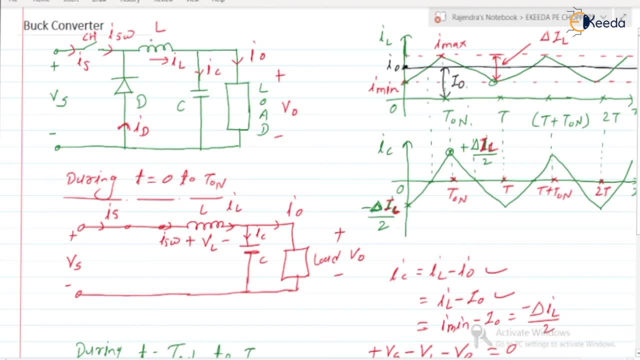 okay. So if you check when switch is in the on state, inductor stores the energy. So current go on increasing from IM into MX, okay. And when switch is in the off state inductor releases the energy. So if you check at all the time, at all the time, 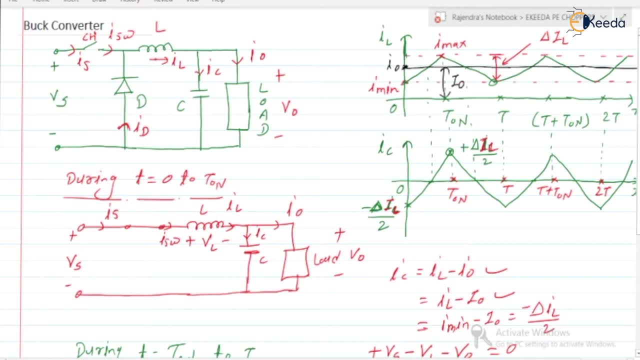 the current flows through the load, it will be non-zero. only Current flows through the load because for one time or during zero to T1, current is flowing from source towards the load And during the when the switch is in the off state at that time, due to the inductor. 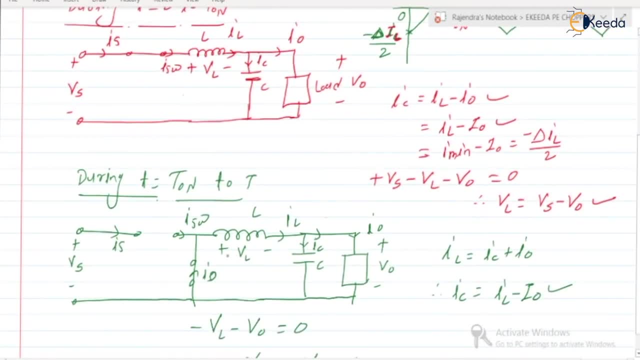 due to the inductor. yes, here, inductor is releasing the energy. means what Inductor current will be flowing right through the load. Are you getting the point? Okay, So this is about the simple operation of the buck converter. Now, as long as the converters are, 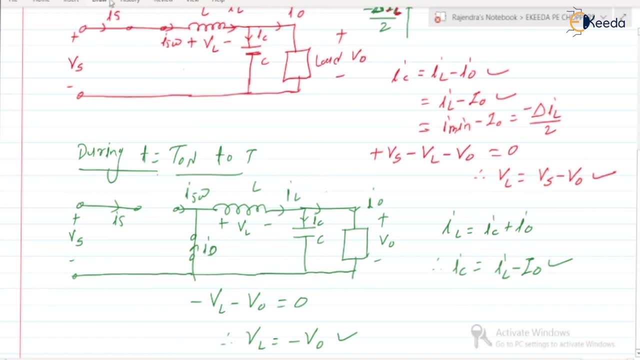 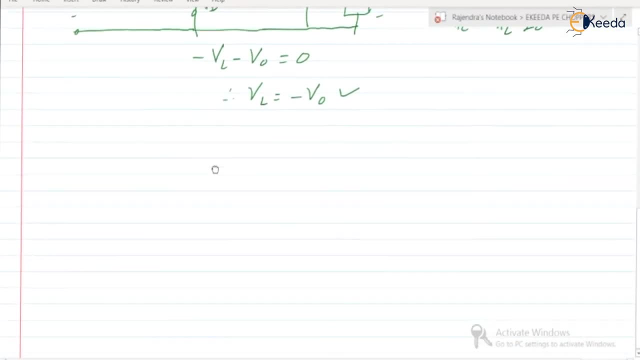 considered okay in the converter circuitry we are going to derive. we are going to derive the 14 expressions, right, 14 different expressions. okay, I am saying 14, 1, 4 different expressions because they have asked the number of questions on these expressions in the previous. 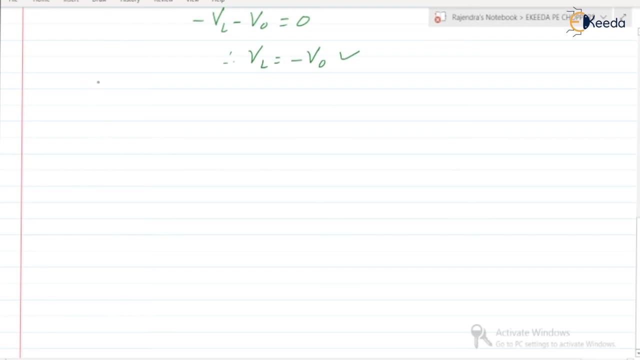 GATE and IES examinations. okay, So we are going to derive the following parameters right following parameters, following parameters: okay, So first we are going to find when switch is on, then find VL and IC. When switch is on SW, switch is SW is on right, then find. 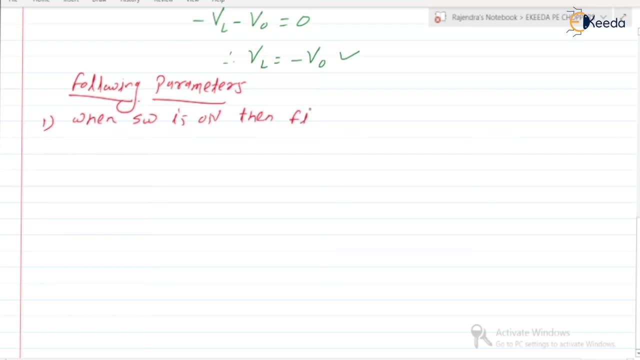 then find, yes, VL and IC. voltage across inductor and current flowing through capacitor. that is the IC, okay. Second, when switch is off: when switch is off, then find, then find, yes, VL and IC, VL and IC. okay. So here, whatever we have found right. 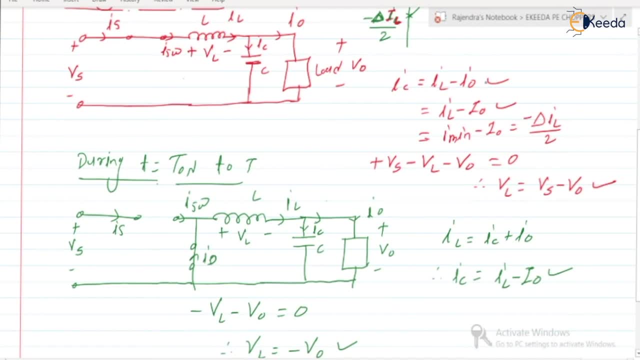 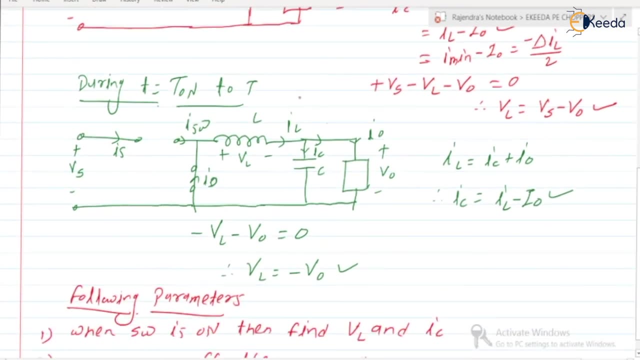 whatever we have discussed here, okay, when switch is in the on state, we have calculated IC, right, we have calculated, we have derived the written, the expression for VL. When switch is in the off state, right, so at that time also we have written IC and again we have written the. 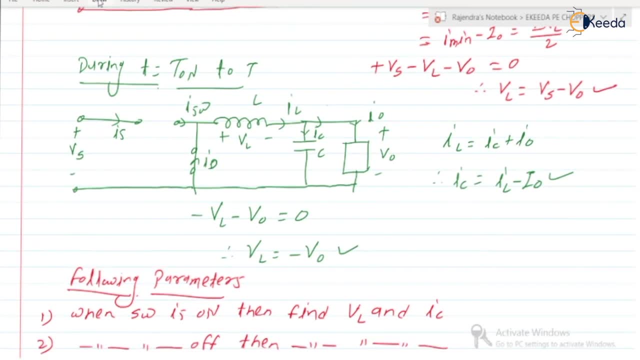 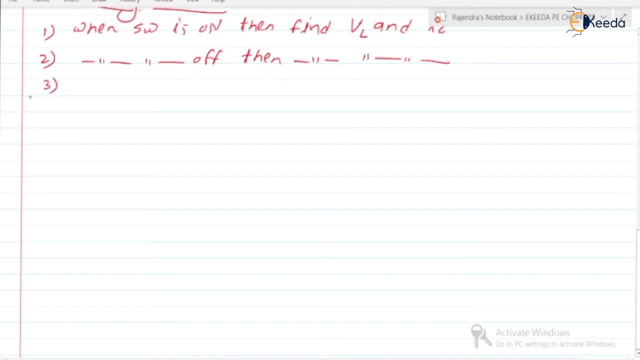 VL as well. okay, So these are the first two steps. The third parameter, right, third parameter. we need to find Third step. third one: it is volt, second balance. okay, We need to write volt, second balance equation. 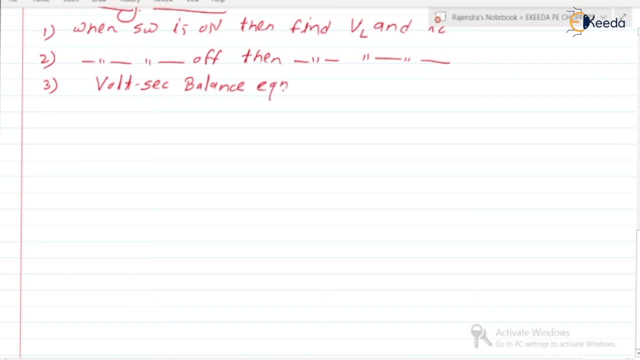 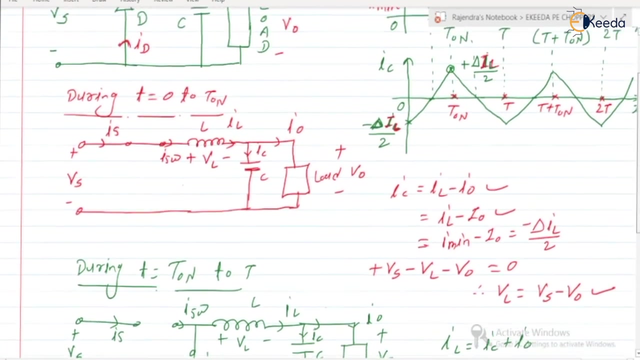 volt second balance. equation right. Fourth one: ampere second balance. ampere second balance- okay. ampere second balance- okay. So please try to understand what is a volt second balance- okay, Volt second balance is nothing but right if you check. 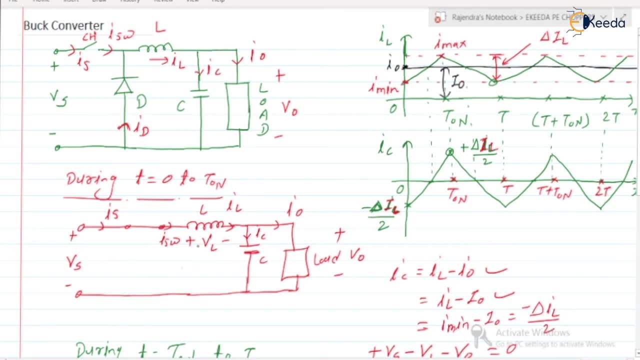 if you check, yes, when switch is in the on state, inductor is restoring the energy right. So current flow to the inductor is changing from I min to I max. right means when inductor stores the energy current is increasing from I min to I max. Again when switch is in the off state. 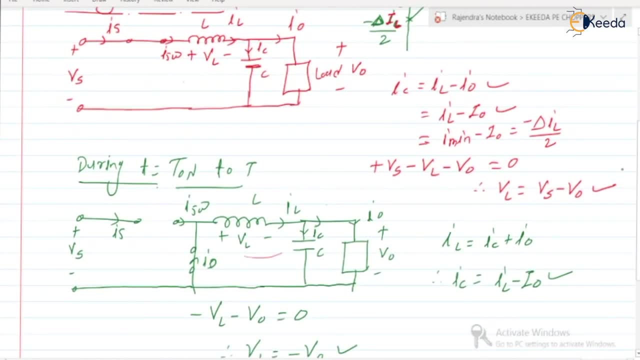 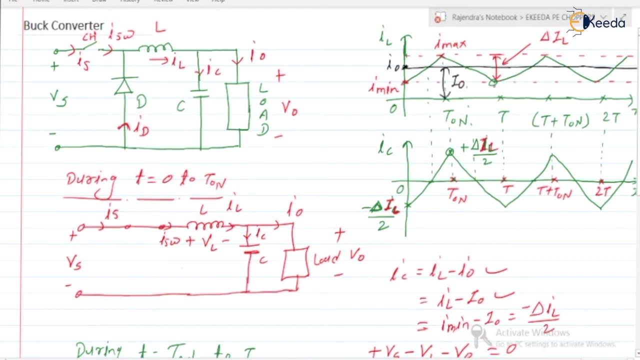 at that time the inductor is releasing the energy, inductor is releasing the energy right. So at that time the voltage, sorry the current flow to the inductor, it go on decreasing from I max to I min. okay, So again for the next cycle, that is, for next on time, it is again. 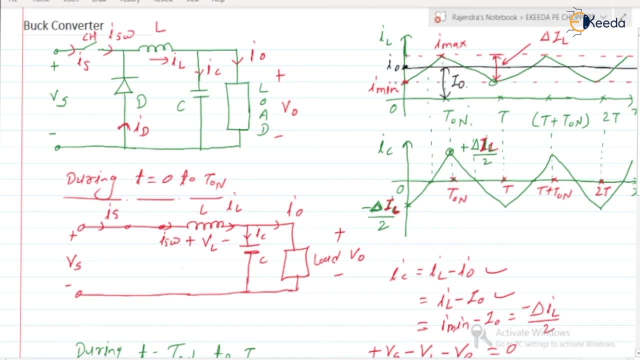 increasing from I min to I max. So if you check, before the starting of the first cycle the current was I min and at the end of the first cycle again the current is I min. So can we say that whatever the energy stored by the inductor is equal to energy released by the inductor? 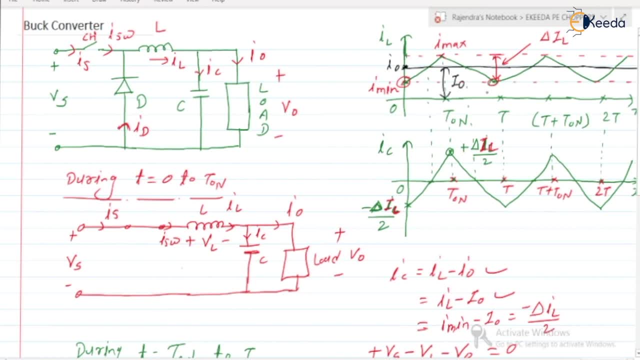 very, very important. and energy stored by the inductor is equal to energy released by the inductor. and in the case of inductor, what is the energy? V into I into time. energy is power into time. So voltage across inductor into current, flowing through the inductor into time. So 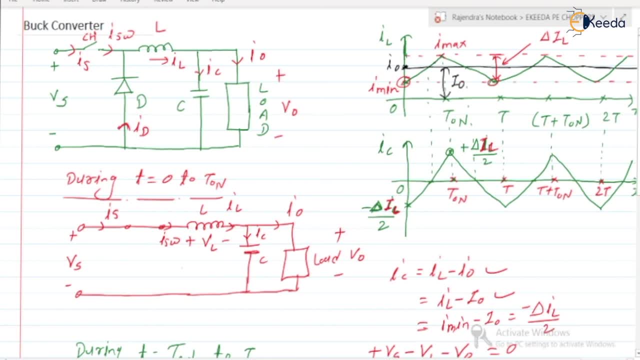 if you check current flowing through the inductor during, or the average current flowing through the inductor during, 0 to t on is same as that of the t on to t, because it is again linear. I min to I max, I max to I min. So what is the average energy? Average energy, will be sorry. average current. 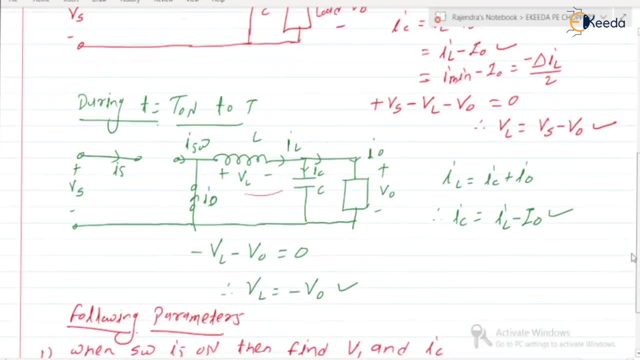 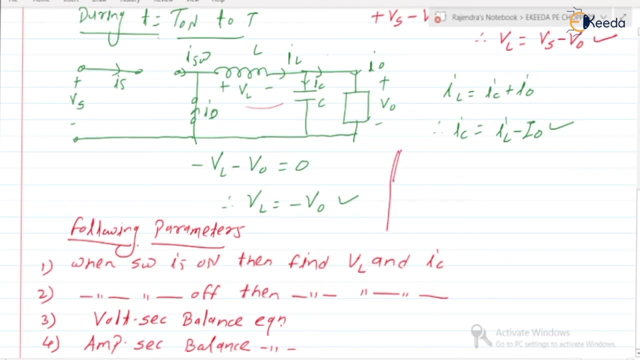 average current is same. So at both these sides it will be getting cancelled and we will be getting only volt. second balance equation: Are you getting the point right? Because in the case of inductor- I am writing In the case of inductor- energy stored by the inductor, energy stored is equal to what energy? 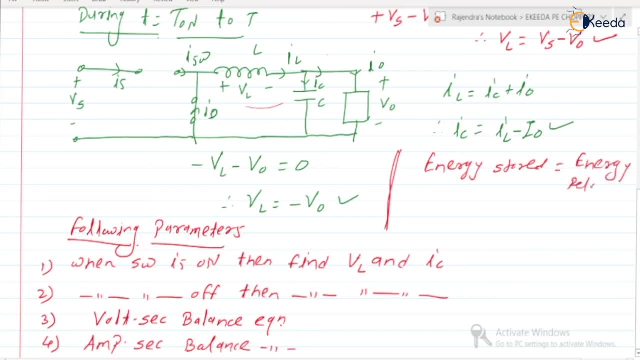 released is equal to what energy released. What is the energy stored? Energy stored is V? L into I L into time. Time is t on. This is doing t on only What is the energy released? V L into I? L into t minus t on. Okay, But what is the average? 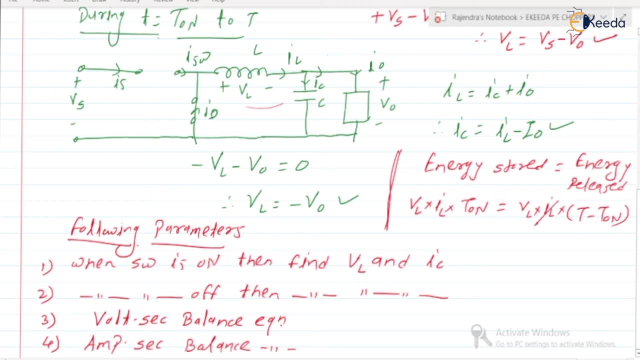 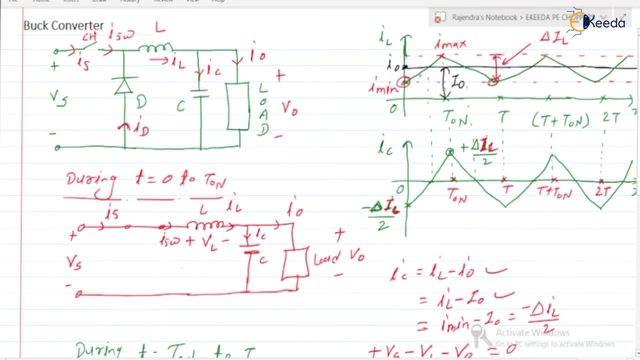 Energy during t on average current during the t on and t off it will be same. So I L, I L will get cancelled. because what is the average when the current is increasing from I min to I max? What is the average value? It is I min plus I max by 2.. Suppose we are having the current which is 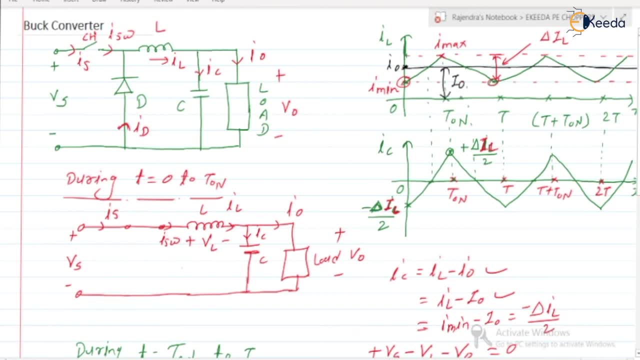 increasing from 0 to 2 ampere. Then what is the average value? Average value will be 1 ampere. How to find the 1 ampere? It is a 0 plus 2 divided by 2, right? So that is what the 1 ampere. If the 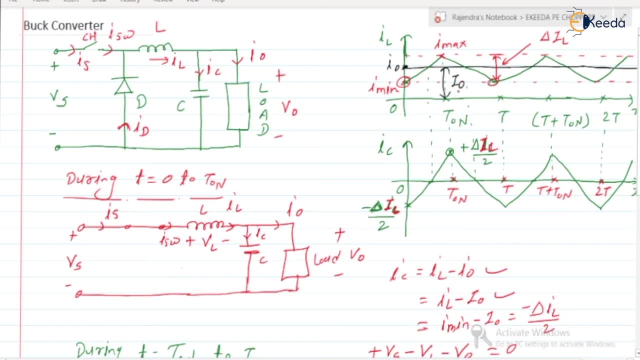 current is increasing from 1. if the current is increasing from 1 to 2, then what is the average value From 1 to 3 ampere, right From 1 ampere? suppose this is 1 ampere, This is a 3 ampere, Then how? 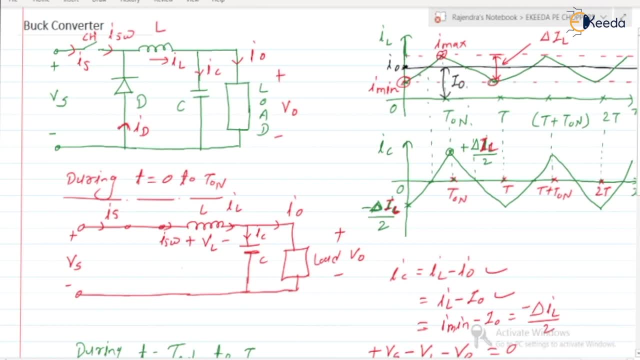 what is the average? It is a 2 ampere. How to find that? 2 ampere, 1 plus 3 divided by 2.. That is a 4 by 2 means 2 ampere. Okay, So similarly average here is I min plus I max by 2.. Similarly here: 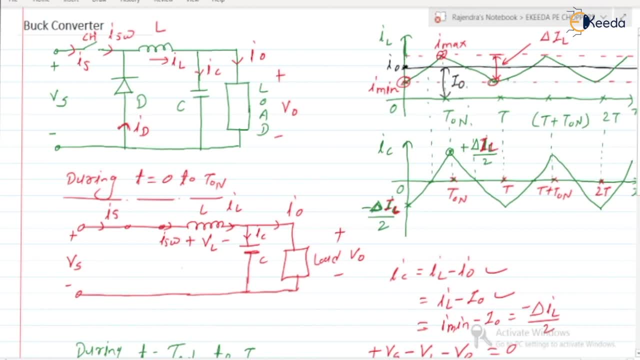 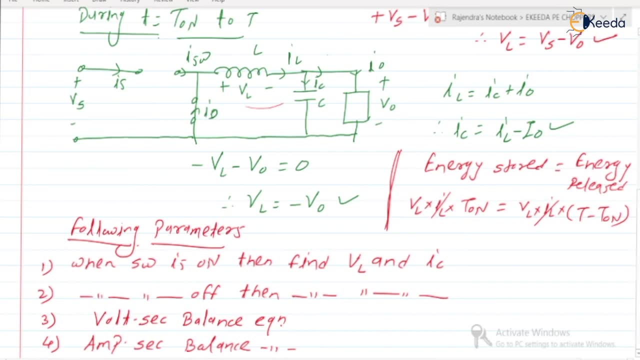 inductor average current is I max plus I min by 2.. So that is why the average current will be same in both the cases, during t on, during t off. So that is why it is like a whole second balance equation, Okay, Whole second balance equation. Similarly, 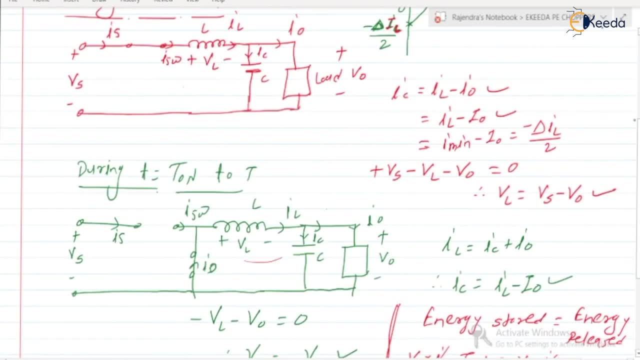 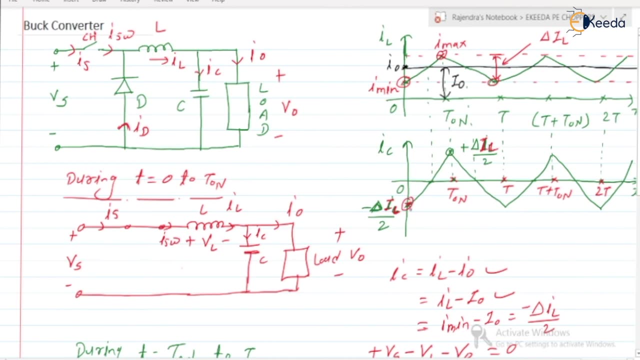 ampere- second balance equation. Ampere- second balance equation. So if you check in the case of capacitor, initially, at the very first or at the beginning of the cycle, the current was minus I L by 2. right Again after the completion of the first cycle, the current is at the same value. 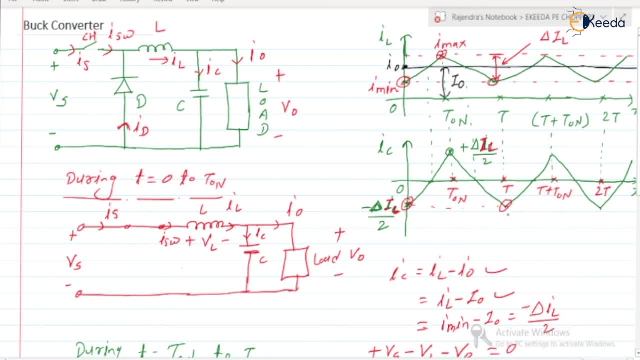 that is a minus delta. I L by 2 only. Is this clear, Okay? So therefore here can we say that whatever the charge is stored by the capacitor, the capacitor releases the same charge. Okay, When switch is in the on state, at that time the capacitor go on storing the charges When switch is. 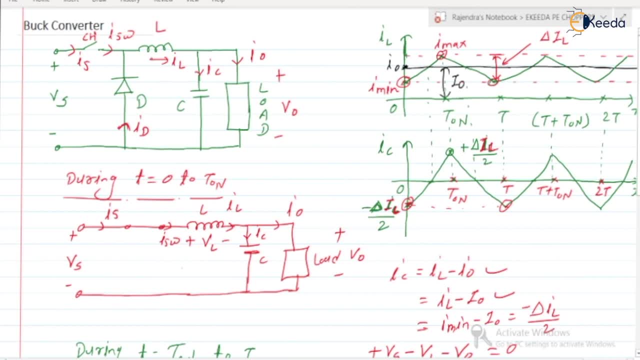 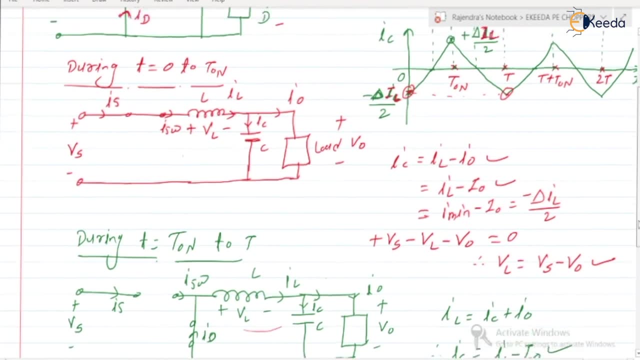 in the off state. when switch is in the off state, then diode conducts right, inductor releases the energy. at the same time, capacitor also discharges Right, So capacitor also discharges. Is this clear? Okay, So therefore, in the case of capacitor, charge stored is equal to charge. 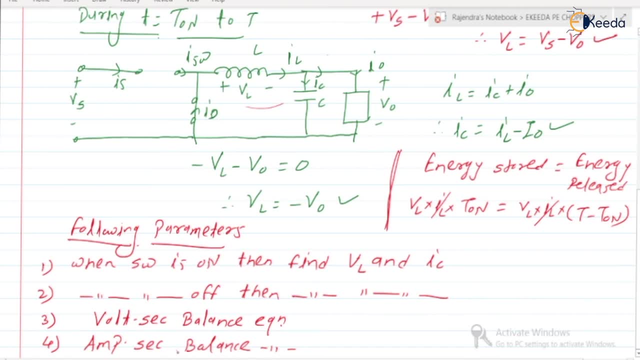 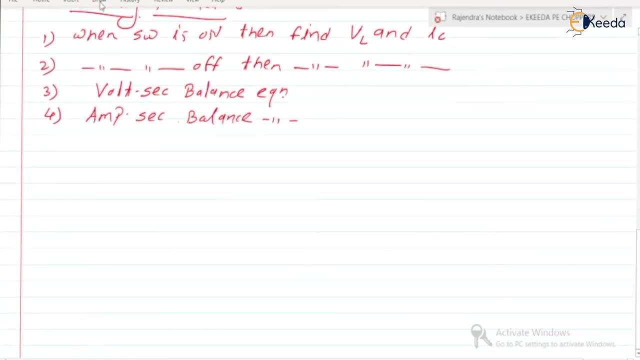 released. What is the charge? Charge is nothing but the current into time, Right? So that is why it is the ampere. second balance equation. Okay, Next fourth or sorry, fifth term we are going to write is: yes, the fifth term we are going to write is: ripple in inductor current. 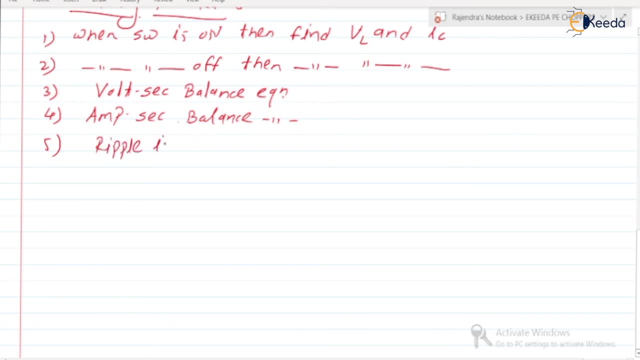 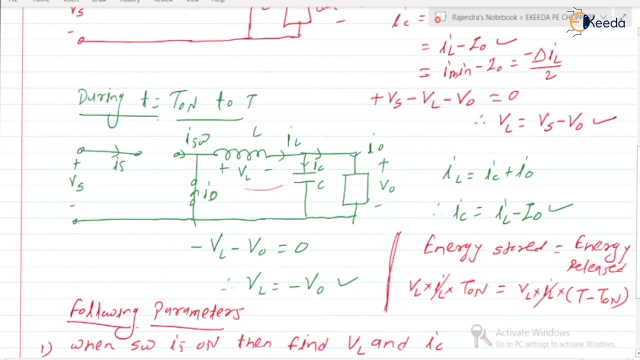 Ripple in inductor current. Ripple in inductor current, Inductor current Right, That is nothing but the delta I L Right. Delta I L Okay Is nothing but change in the inductor current, Change in the inductor current. So if you check, the inductor current is changing from I min to I max. So what is the 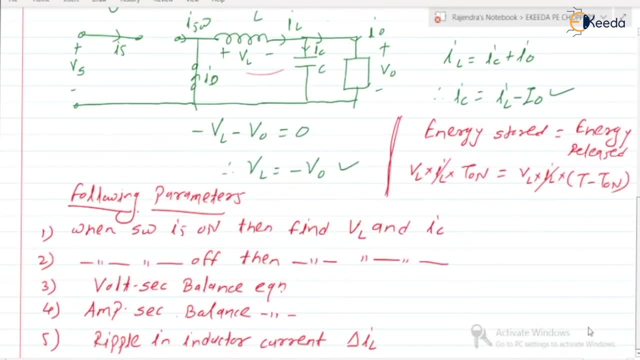 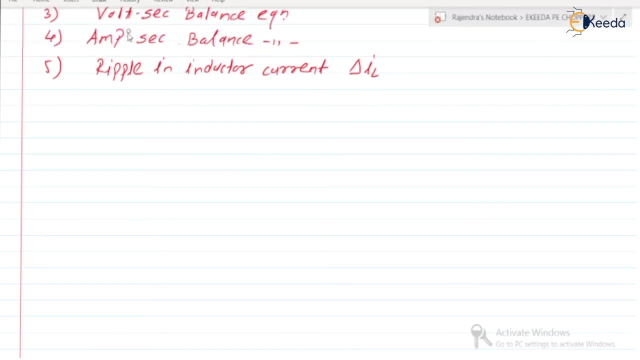 ripple. It is I max minus I min. I max minus I min. That is the ripple. Okay, Next sixth parameter. we are going to write Sixth parameter: Yes, it is I L max For the maximum inductor current. they want I L min. Okay, I L max and I L min. Okay, It is the I L max. and next one is the I L min. Right. Next parameter走. 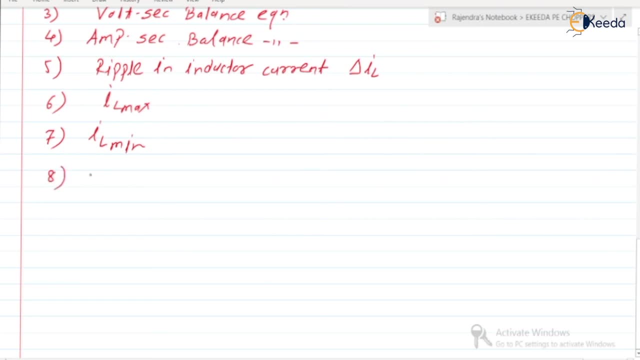 okay. eight parameter: is source current. is source current: average value of the source current. we are going to write, okay. ninth parameter: we are going to write or write the expression or derive the expression: is the switch current, switch current, switch current, okay. average and rms: average and rms. 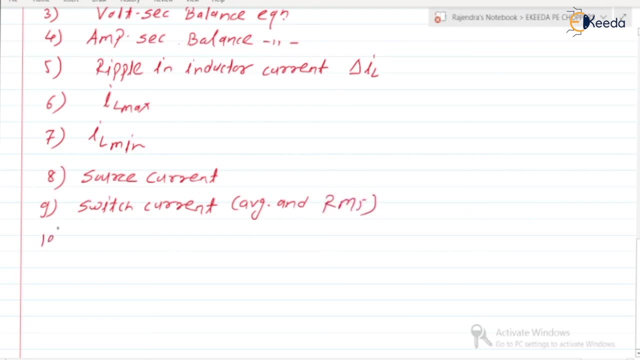 okay, 10th parameter, we are going to write diode current. diode current: yes, it is the average and rms. rms and average value of the diode current. right 11 number is ripple in capacitor voltage. ripple in capacitor voltage or it is also known as if you check capacitors connected in parallel with the load right.